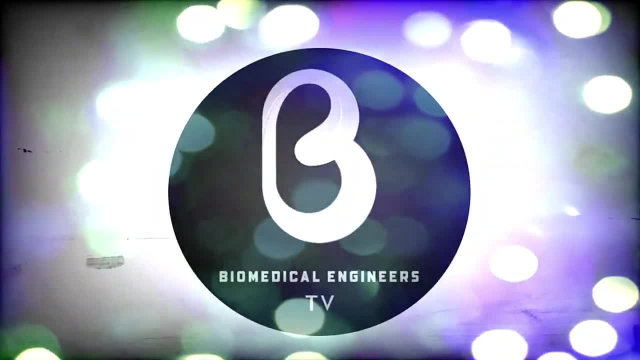 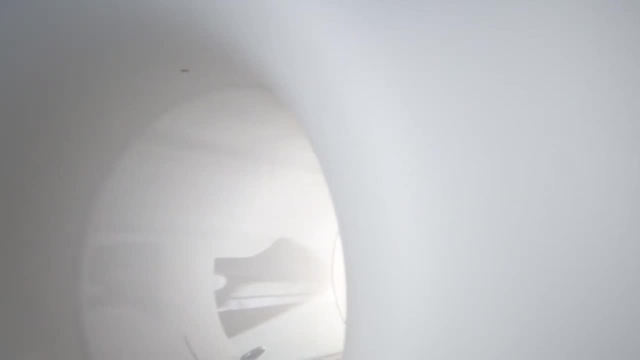 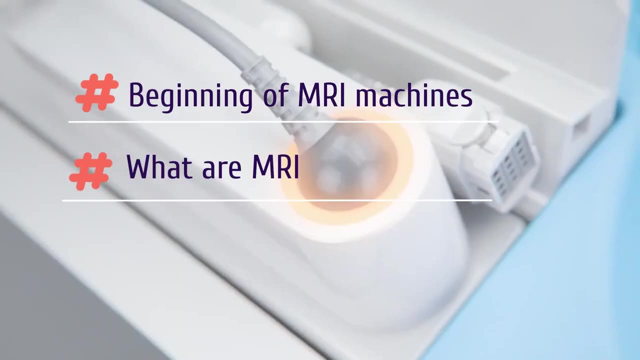 Hi, welcome to Biomedical Engineers TV. In this series we will look into MRI machines. In this video we will cover the beginning of MRI machines. what are MRI machines and the types of MRI machines. If you like our videos, do subscribe to the channel and give. 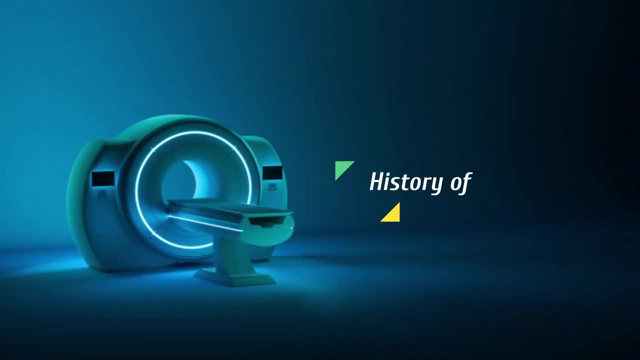 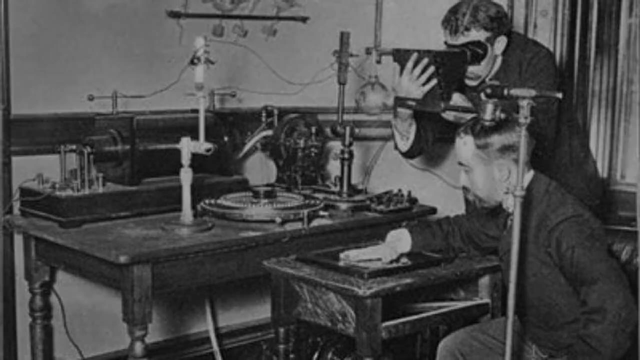 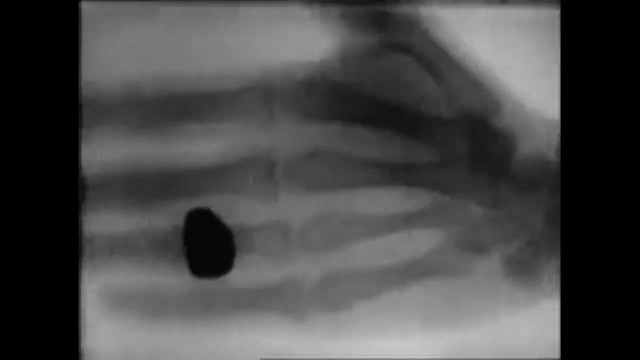 us a thumbs up. Let's begin with the history of MRI machines. A magnetic resonance imaging machine, better known as an MRI, has a long and complicated history, beginning in 1945.. It all started when Swiss physicist named Felix Bloch conducted an experiment regarding a new method of nuclear 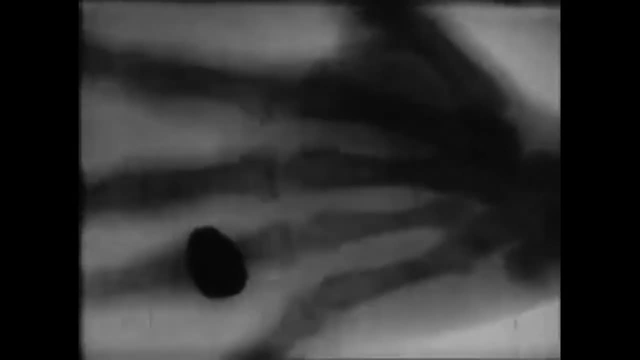 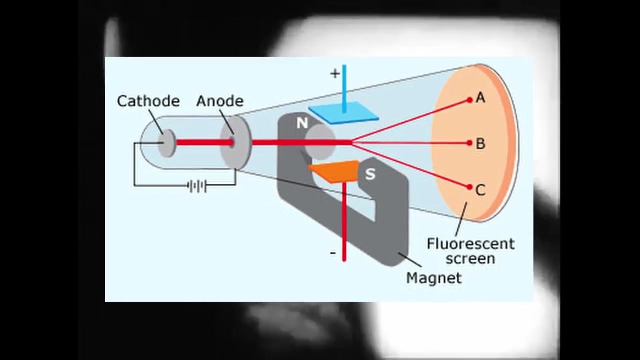 induction – a study of nuclear moments in solids, liquids or gases. It was by pure chance that, at this same exact time, the same experiment had been made by Edward Mills Purcell and his collaborator Dr Robert M Purcell. 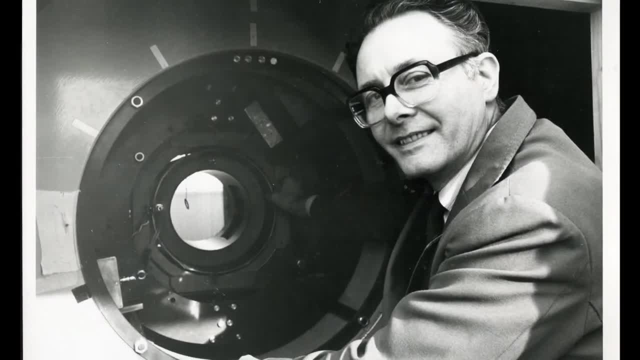 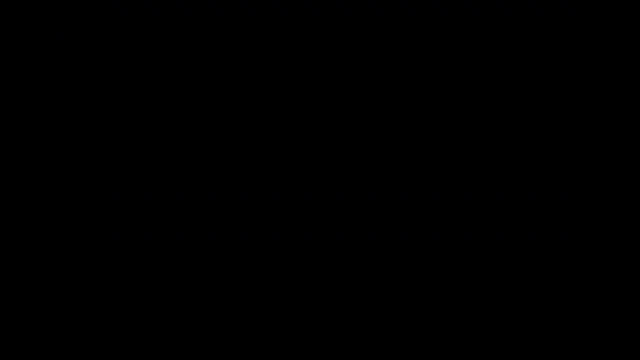 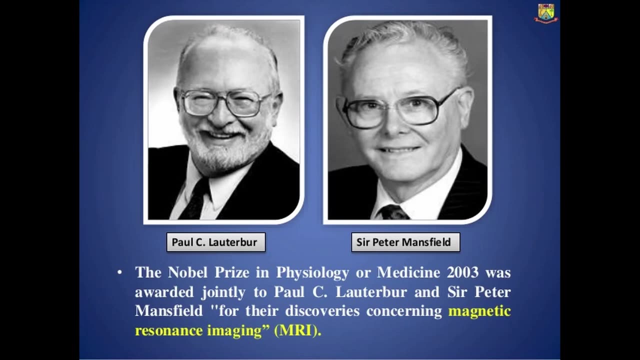 M Purcell was an Illinois native with a degree in electrical engineering and together both Purcell and Bloch won the 1952 Nobel Prize for Physics for their published papers on nuclear magnetic resonance, or NMR, which is the science behind the MRI. 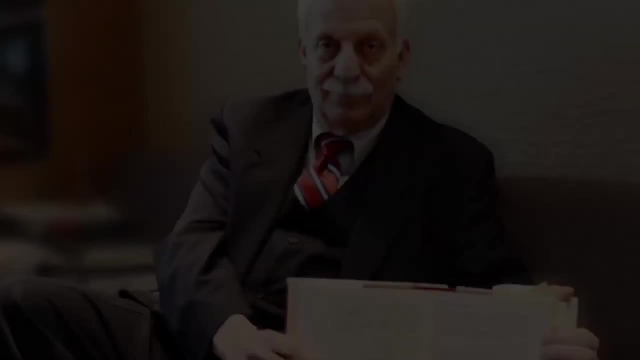 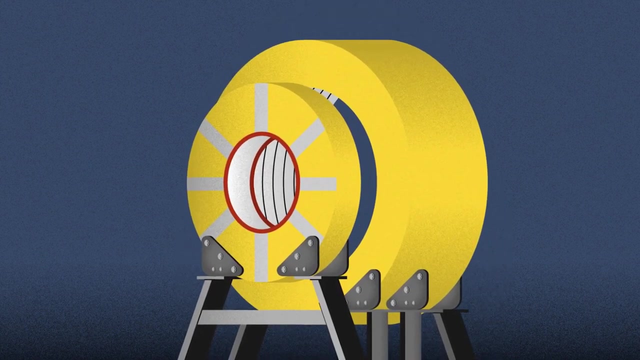 A year later, Raymond Damadian created the first full-body MRI machine and the first MRI body exam was operated on a human. It took almost five hours to produce one image. In the years following the first MRI machine, full-body exam technology has come a long. 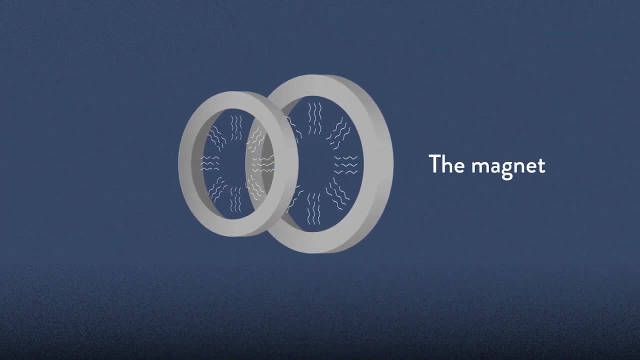 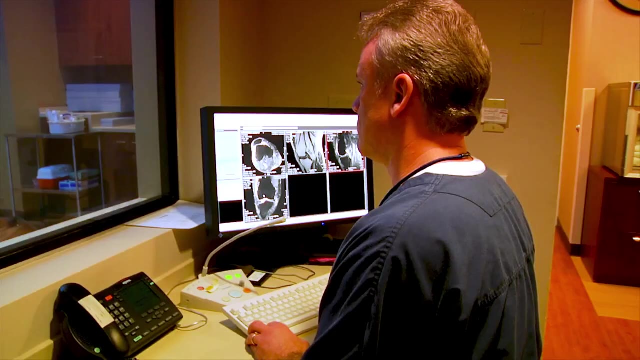 way. The machine uses magnetic fields to scan the patient and then sends the signals back to be converted into images by a computer. Today, an MRI scan can take anywhere from 10 minutes to over two hours, depending on the size of the area being scanned. 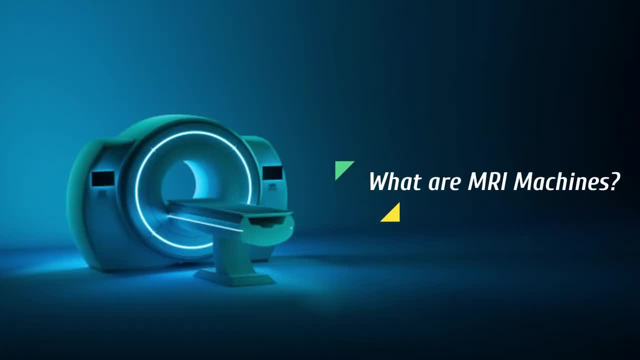 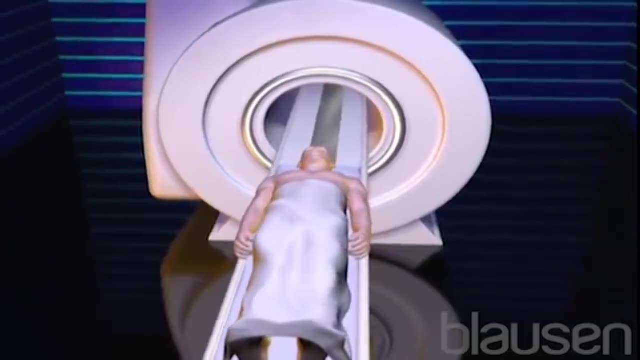 Let's know about. what are MRI machines? During an MRI scan you lie on a flatbed that's moved into the scanner. Depending on the part of your body being scanned, you'll be moved into the scanner either head-first or feet-first. The MRI scanner is operated by a radiographer. 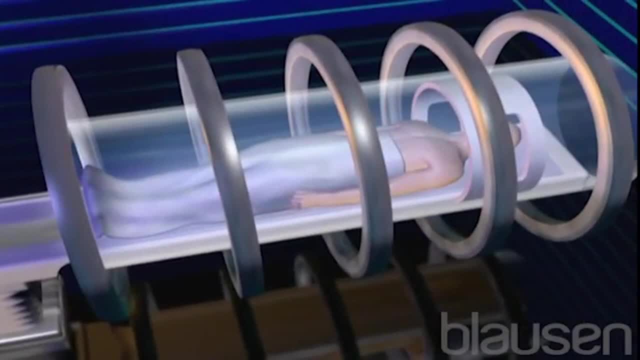 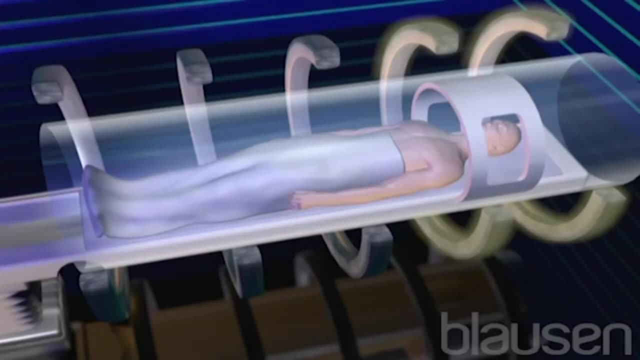 who is trained in carrying out imaging investigations. They control the scanner using a computer which is in a different room to keep it away from the magnetic field generated by the scanner. You'll be able to talk to the radiographer through an intercom and they'll be able to. 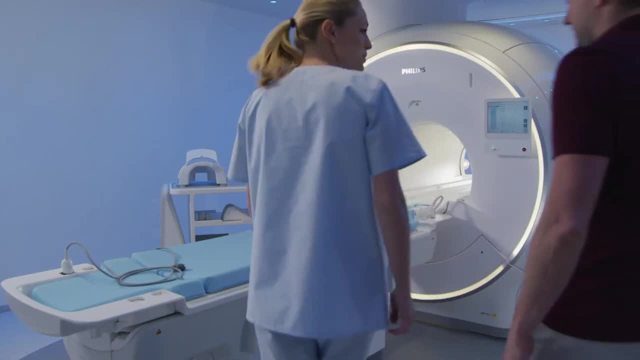 see you on a television monitor throughout the scan. At certain times during the scan, the scanner will make loud, loud noises. The scanner will be able to see you on a television monitor throughout the scan. At certain times during the scan, the scanner will make loud. 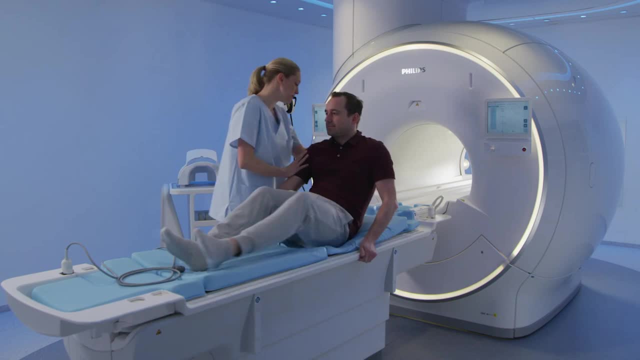 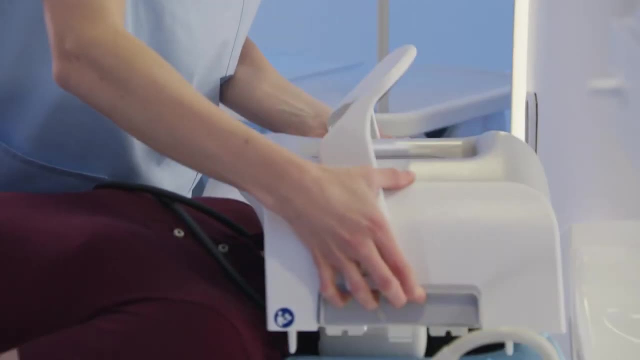 tapping noises, A coil might be placed around the part of your body being scanned, such as your head, knee or abdomen. This coil is really a special radio receiver that improves the picture and is usually contained in hard white plastic. If the coil begins to become 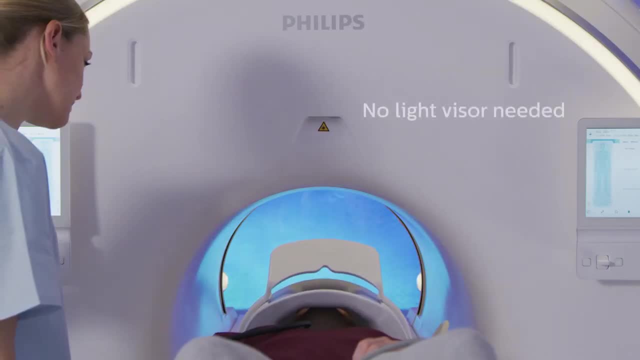 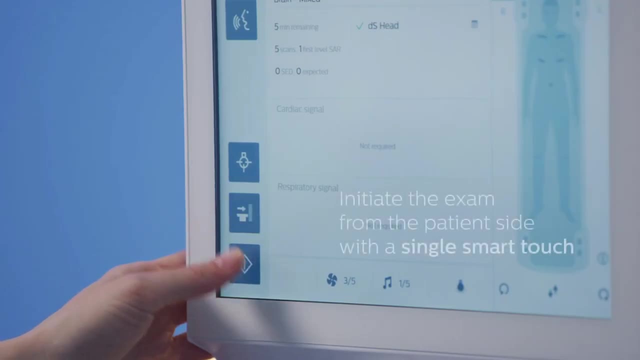 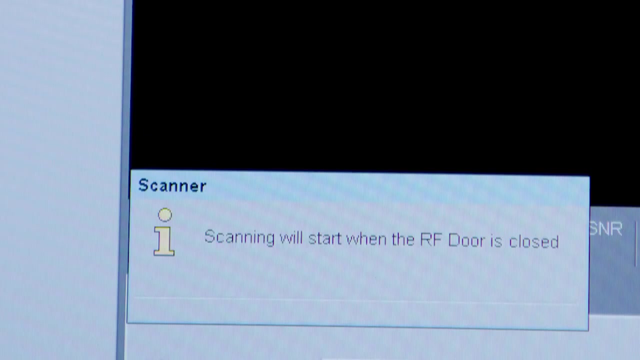 uncomfortable during the scan, tell the MRI technologist. This is the electric current in the scanner coils being turned on and off. You'll be given earplugs or headphones to wear. It's very important to keep as still as possible during your MRI scan. The scan lasts 15 to 90 minutes depending on the size of the area. 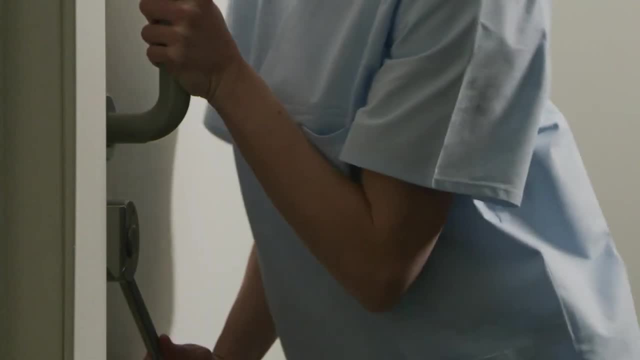 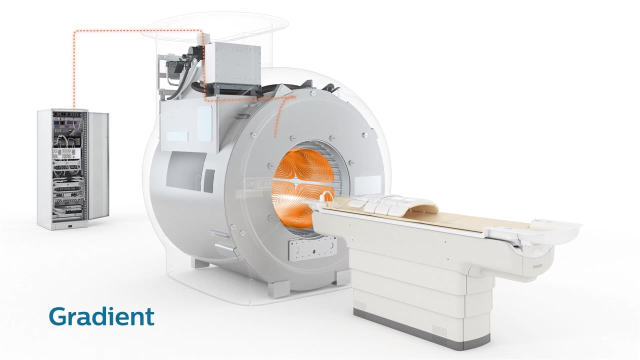 being scanned and how many images are taken. Let's see the different types of MRI machines. A magnetic resonance imaging or MRI machine is a sophisticated medical imaging and diagnostic device. They create a low-level magnetic field which causes a specific reaction inside the atoms of the body, The atoms inside each type. 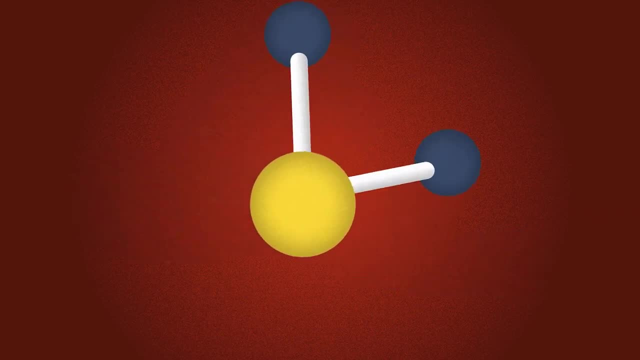 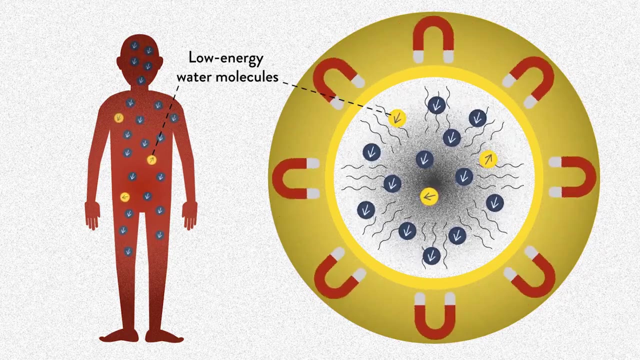 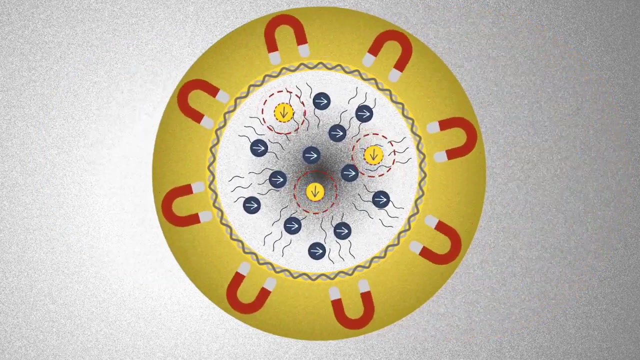 of tissue in the body react in different ways. The computer hooked up to the scanner senses these different reactions and then turns what it senses into a visual representation of internal functioning of the patient's body. In the past, all MRI machines not only worked the same, but also looked the same. Today, though, there are four different types of 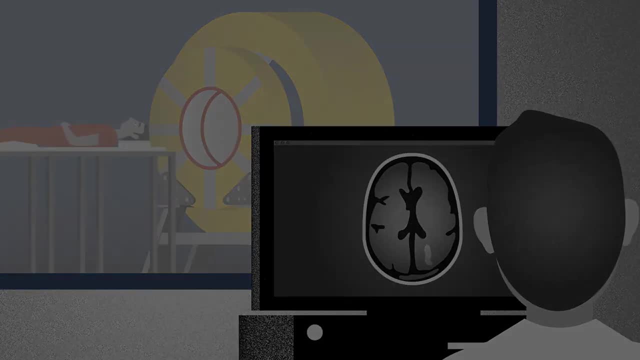 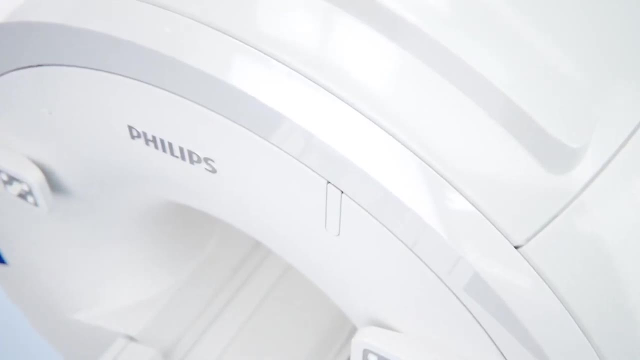 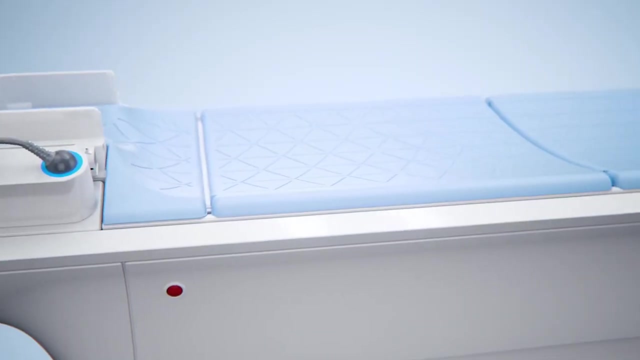 MRI scanners available to patients. The first type of MRI machine is the traditional closed MRI. A closed MRI machine is a large tube that a patient lies in. This style of scanner almost always produces images that are of very high quality. Patient comfort in these machines is sometimes a problem. 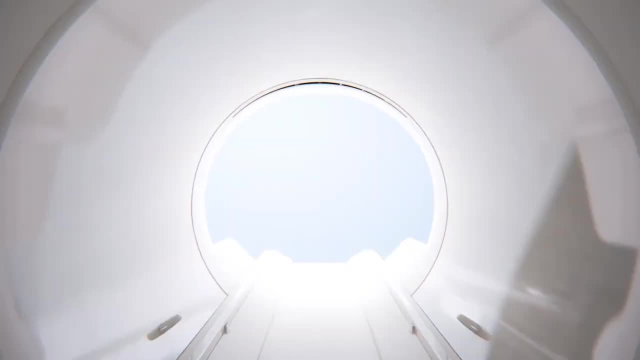 The small tube that a patient must lay in can cause a patient who is claustrophobic to panic. The MRI machine requires the patient to lie very still. Someone who is moving around can make scanning almost impossible. The small opening size of some closed MRI machines means 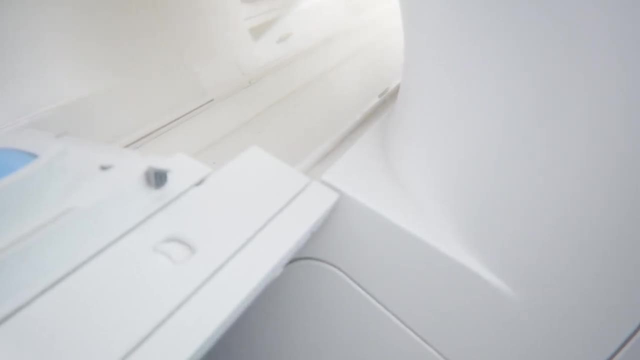 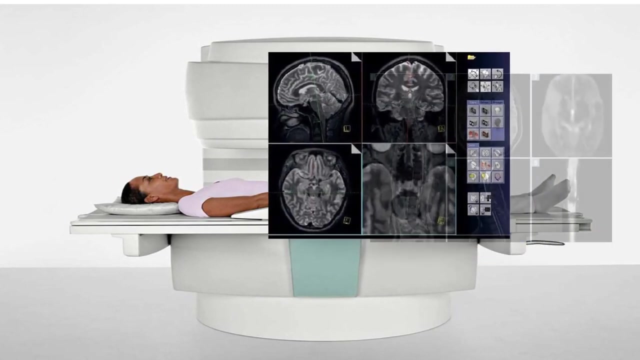 that the overweight patients simply cannot be scanned. The second type of MRI machine is open MRI scans. In an effort to allow claustrophobic patients more comfort and to allow obese patients to be scanned, the open MRI was developed. Older open-type scanners did not produce very good quality images due to a reduced number.